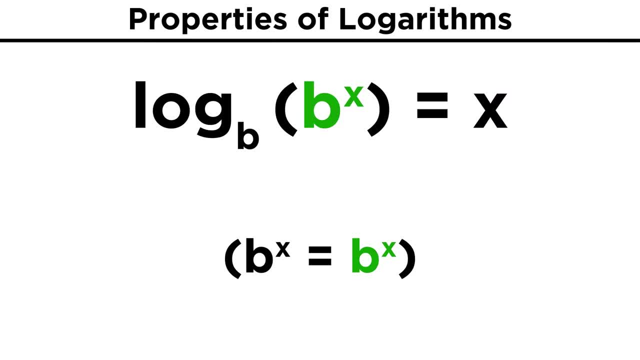 be expressed as: B to the X equals B to the X. So when you see the log of an exponential term where the bases match, it all goes away and we are just left with the exponent: Similarly B to the log, base B of X also equals X, because this log represents the number. 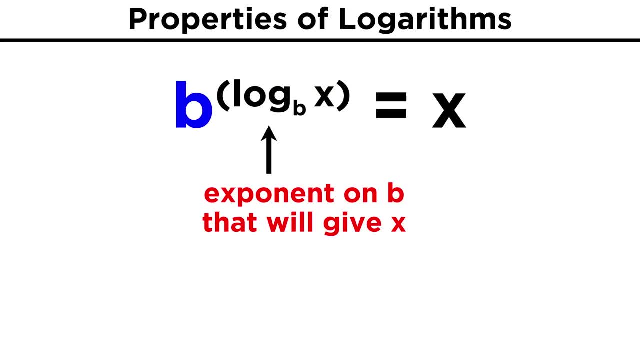 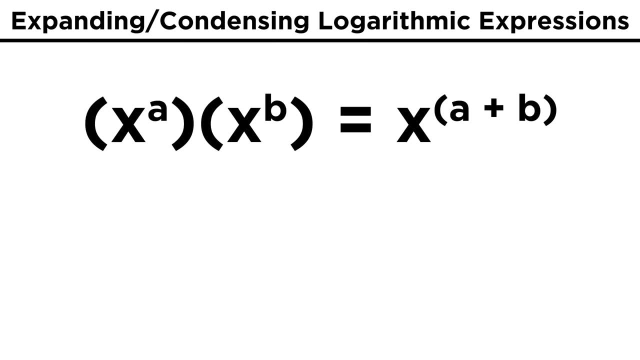 B must be raised to in order to get X. so if B is raised to that number, we must get X. Now let's learn some properties that will allow us to do operations with logarithmic terms. These properties will correspond to properties of exponents that we already know. 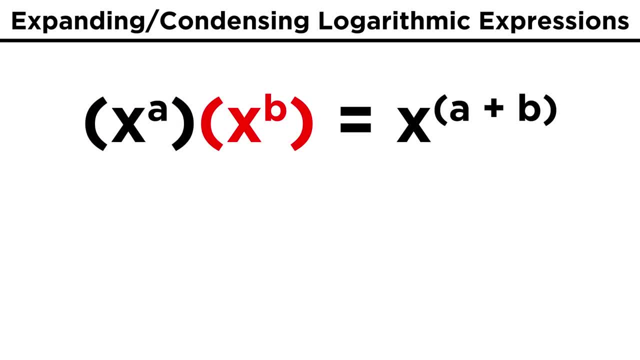 For example, we know that X to the A times X to the B equals X to the A plus B, which allows us to combine terms or split one term up into two, Because logarithms are essentially exponents. then it should follow that for any base, including 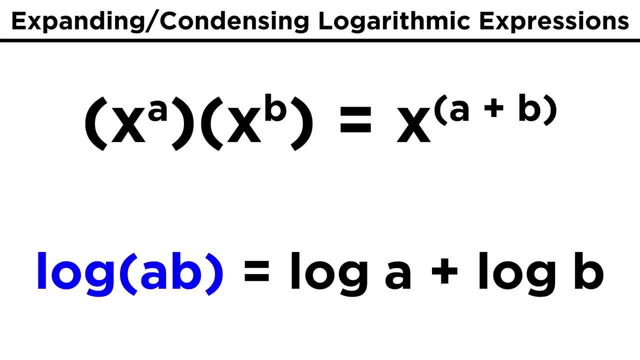 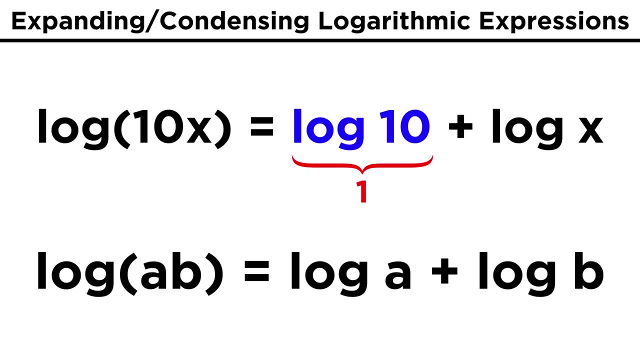 base ten, which we will assume for the time being. log of A- B equals log of A plus log of B. That means we can take something like log of ten- X and turn it into log of ten plus log of X. Log of ten is one, so this becomes log of X plus one. 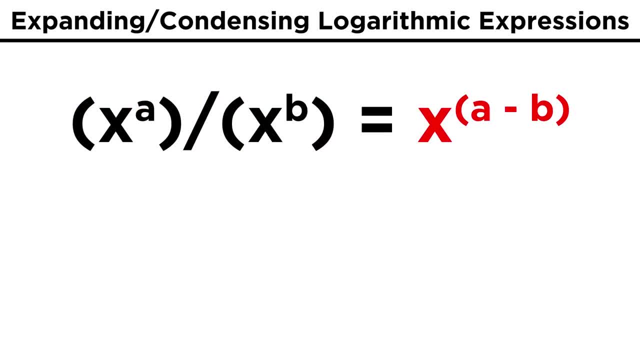 We also know that X to the A, over X to the B, equals X to the A minus B, which again can be used to expand or condense certain expressions. Therefore It is the case: over B equals log of A, minus log of B. This means that with something like log of three, 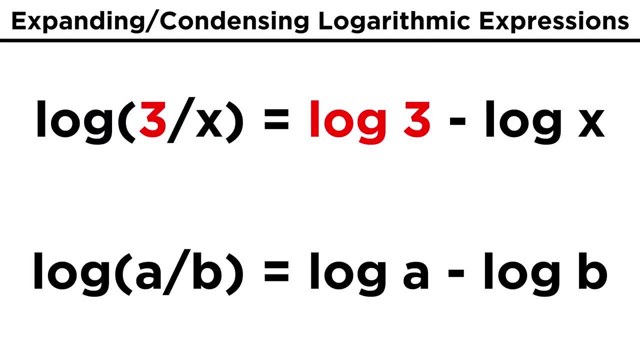 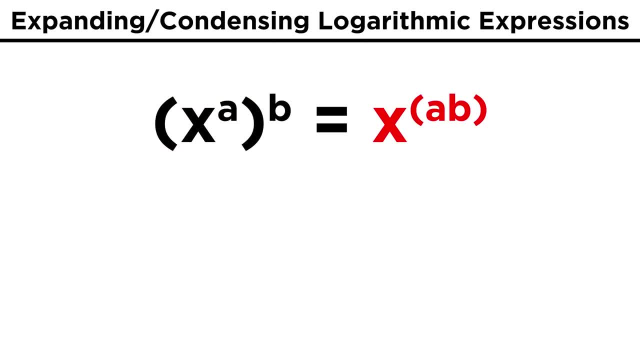 over X. we could express it as log of three minus log of X. Next, we can remember that X to the A to the B equals X to the A times B. The corresponding property for logs tells us that log of X to the A equals A log X. so if we have log X, 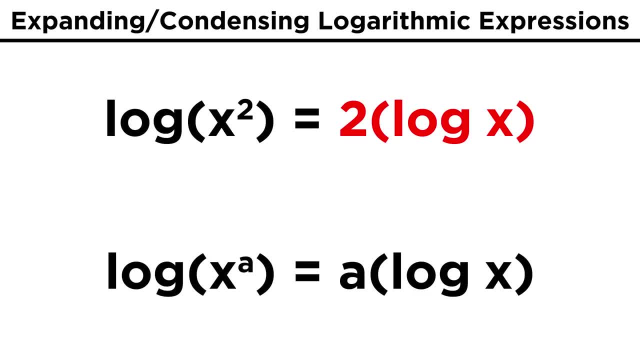 squared, that is the same as two log X. Let's quickly mention that this only applies if the exponent is part of the term that the logarithm is operating on. If we had log of X, quantity squared, that just means log of X times, log of X, just as. 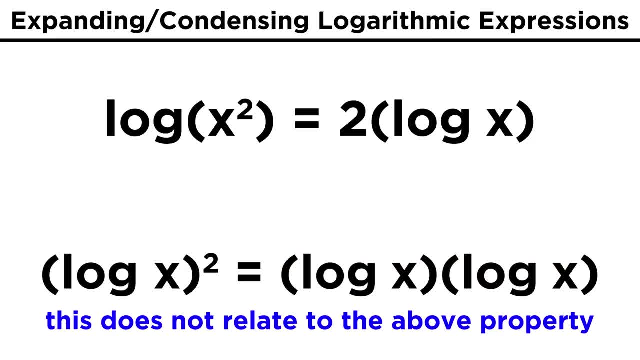 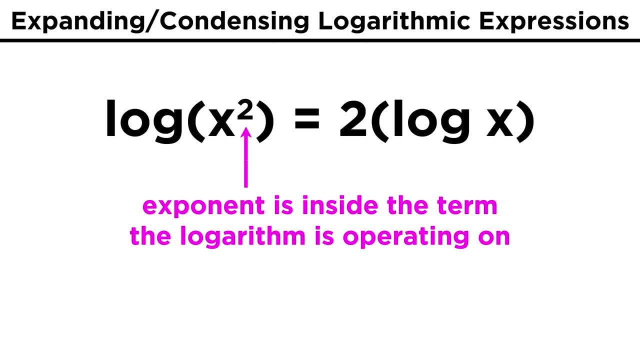 with anything else that we could square. This is not related to the property we are describing. When the exponent is in here on this X term, It means that we are taking the log of X squared and it is in this case that we can pull the. 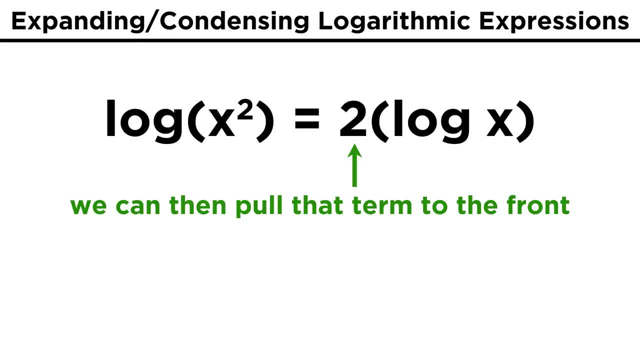 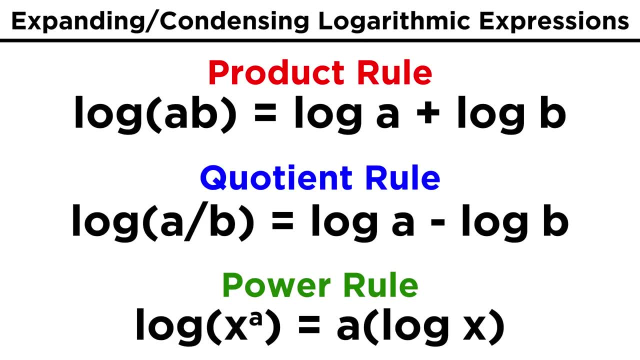 two over to the front and get two log X. So these are the three ways that we can expand logarithmic expressions. They are the product rule, the quotient rule and the power rule. Now that we know these rules, let's practice a bit. 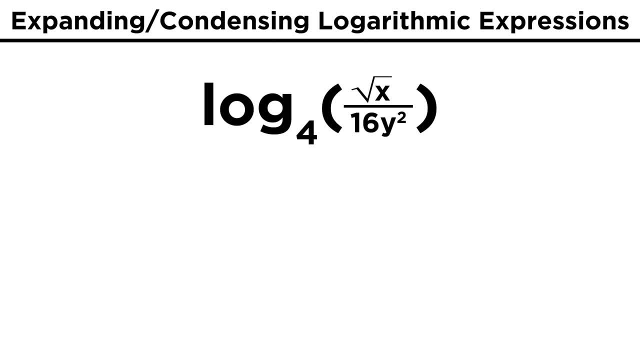 Try log base four of the square root of X over sixteen Y squared. First thing we notice is that we have a quotient. so let's break this into log of root X minus log of sixteen Y squared. This second term has a product, so we can expand again. 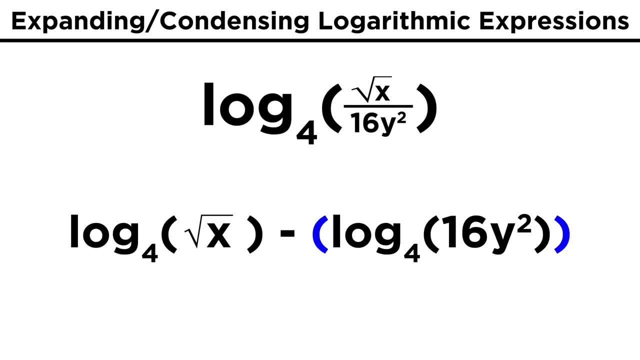 But we have to be careful about our signs. To be safe, let's put this term in parentheses first. After expanding, we get log sixteen and log Y squared. Now to get rid of the parentheses, we have to distribute this negative sign. 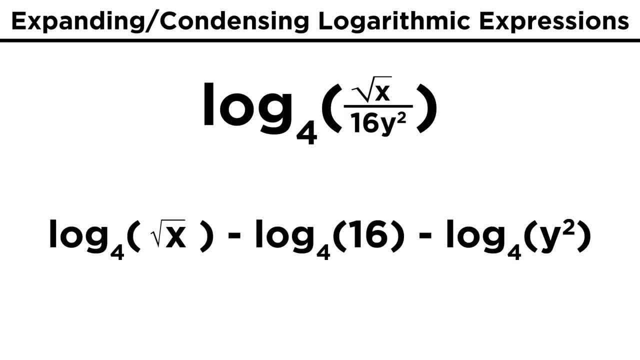 So both of these terms become negative and we are now done with that step. We can actually simplify further. Starting on the left, let's rewrite root X as X to the one half. We know that we can pull exponents to the front, so this becomes one half log X. 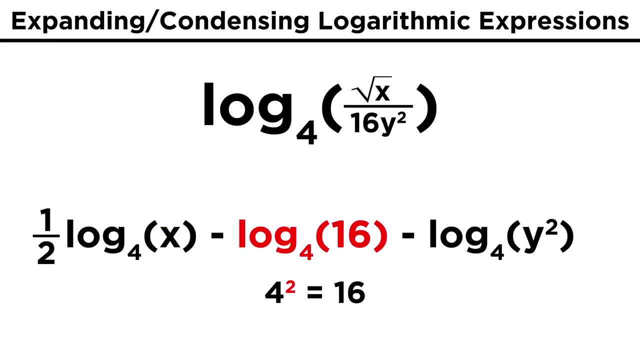 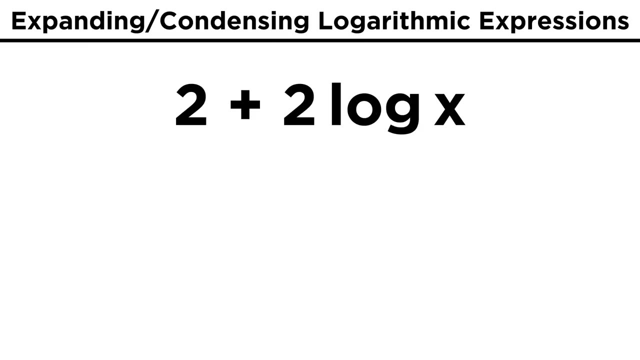 Then log base. four of sixteen is two, because four squared is sixteen, so this becomes minus two. We can pull the exponent to the front on this last term to get minus two. log Y and there is our expanded expression. Just for fun, let's take some other expression and see if we can get it to condense into.